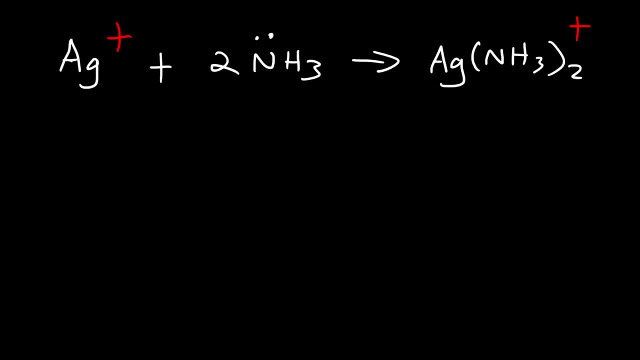 Now what is the coordination number of that complex ion? The coordination number is two because it's attached to two ligand molecules. So this is the ion, or the metal ion, This is the ligand, And here we have the complex ion. 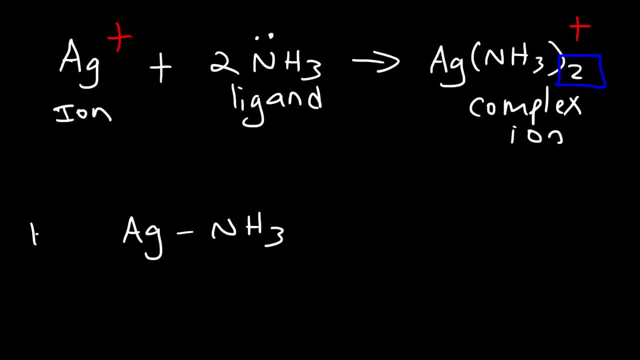 Now for complex ions that have a coordination number of two. the geometry will be linear, as you can see from this particular drawing, And so that's a basic introduction into complex ions. So now let's look at another example: The hexacyanophery ion. 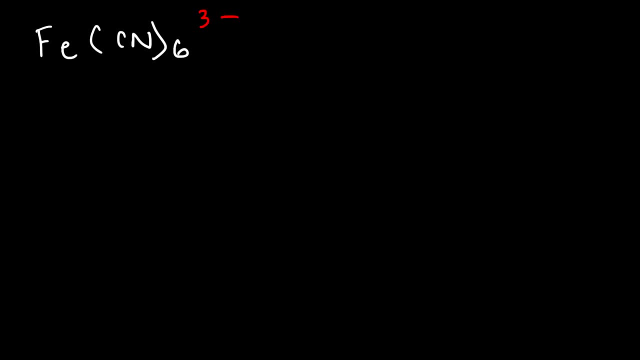 Identify the ligand and also determine the coordination number and the oxidation state of Fe. The ligand in this example it's not a molecule, but it's a polyatomic ion. In this case it's cyanide, which has a Lewis structure that looks like this: 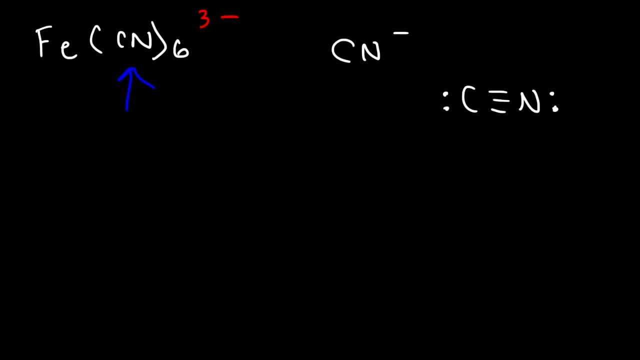 The carbon bears the negative charge Or the negative formal charge. Now the coordination number is basically the number of ligand ions attached to the transition metal cation. So the coordination number in this example is six. Now how can we determine the oxidation state of Fe? 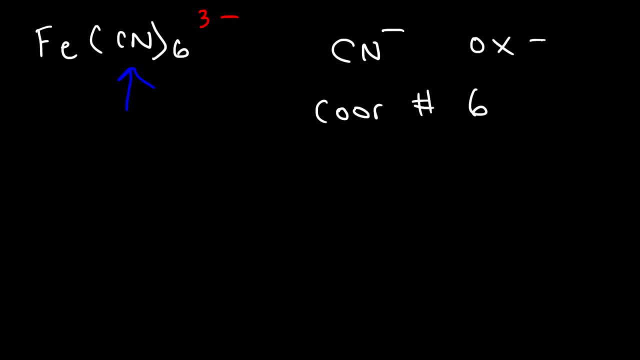 Would you say it's positive, three negative three positive four negative two. What is it? Well, let's write a reaction. So we know that Fe probably has some charge, which we'll call X, And it's going to react with six cyanide ions to produce the hexacyanophery ion. 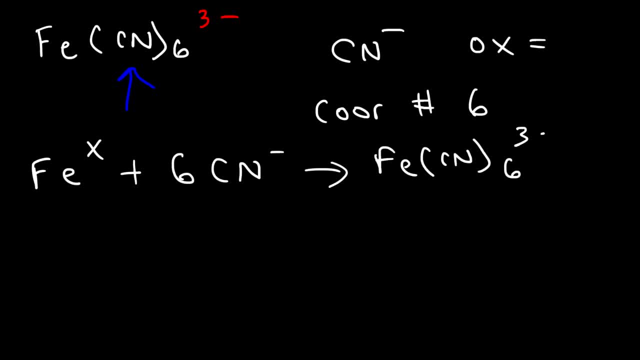 Almost lost the word there. So let's write an equation where the total charge will remain balanced. So Fe has a charge of X, cyanide has a charge of negative 1, but there's six of them, and the product ion or the complex ion has a net charge. 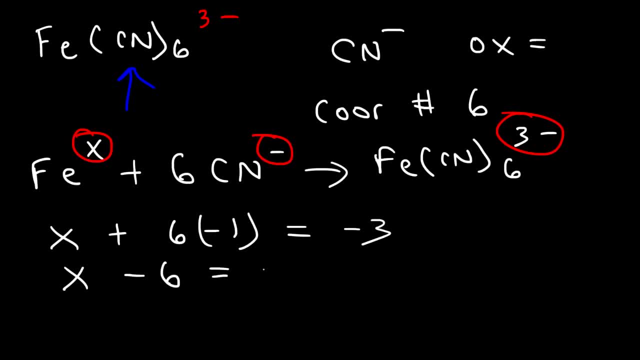 of negative 3.. So X minus 6 is equal to negative 3.. So if we add 6 to both sides, we can see that X is negative 3 plus 6 or plus 3.. So this is the oxidation state of Fe. So Fe has a positive 3 charge. Now there was a guy called Alfred. 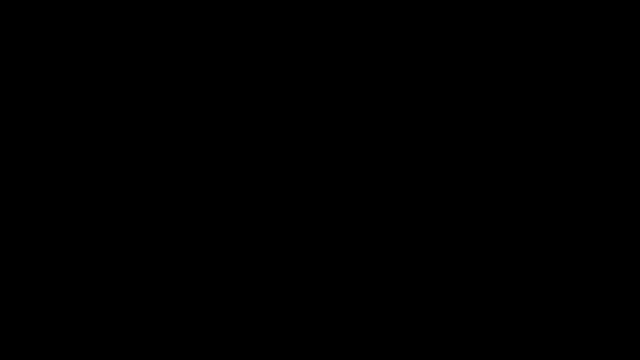 Werner and he came up with a theory for coordination compounds and transition metal ions, And he basically stated that transition metal ions have two types of valence, and that is that the way that these metal cations can combine with other things like ligands and ions, And the two types of valence. 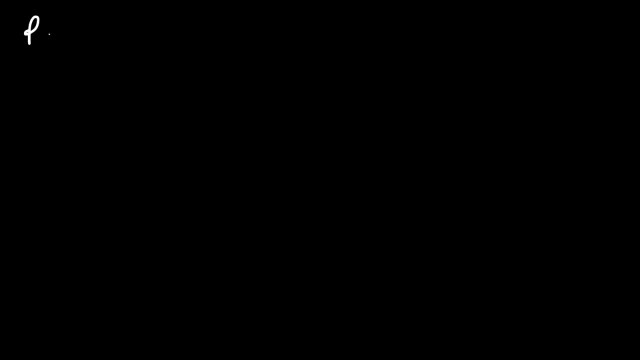 that these metal ions can have is called: the first one is the primary valence and the second one is the secondary valence- Perhaps you've heard of these terms- And, in the case of X, the Fe ion. as it relates to this particular complex ion. What do you think? 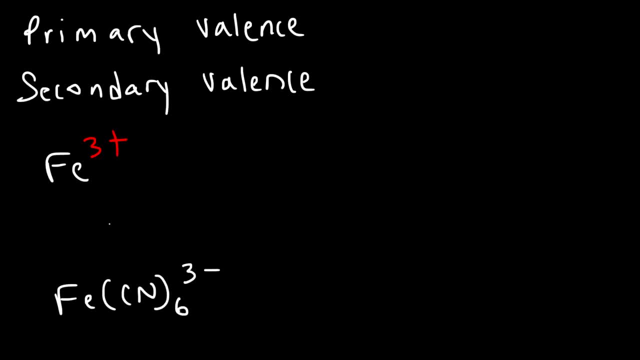 the primary valence and the secondary valence of this transition metal cation is. The primary valence has to do with its oxidation state and thus the way it forms ionic bonds. The secondary valence has to do with the coordination number, and so it relates to how it 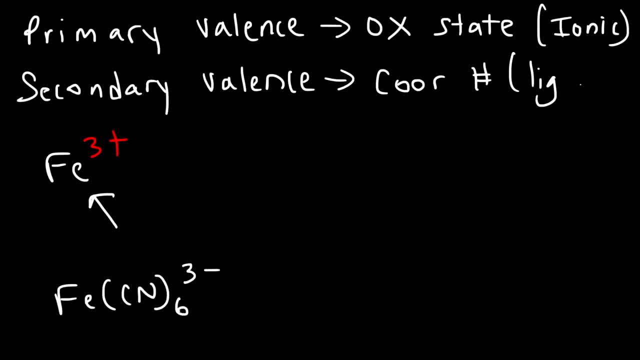 interacts with ligands, And those ligands could be ions or molecules. So in this case the primary valence is positive 3, because that's the oxidation state of Fe, And the secondary valence is 6 because the coordination number is 6.. It could be attached to 6 ligands. Now what type of geometry does the FeCn6 3- ion have? 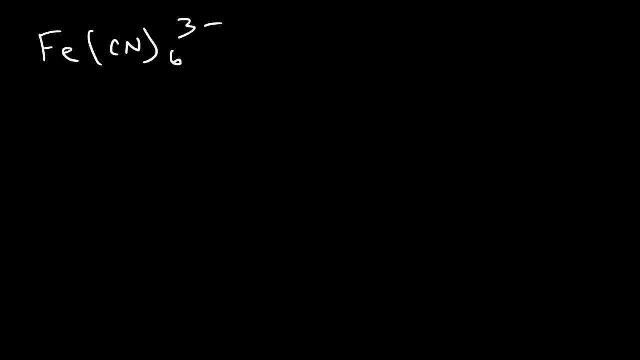 Now, what type of geometry does the FeCn6 3- ion have? If the coordination number is 6, the geometry will be octahedral, And so it's going to look like this. And so that's how you can draw this particular complex ion. And, if you want, 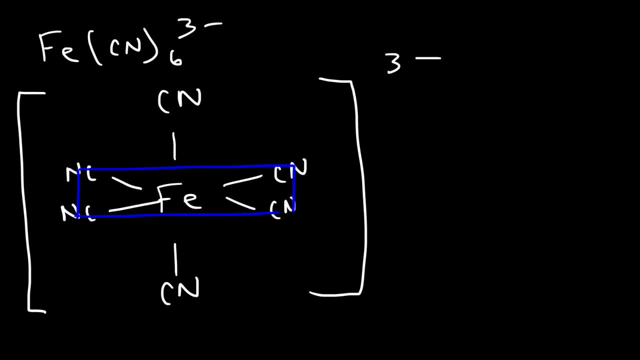 to show the octahedral structure you could. you can make it look like this: So that's the octahedral structure of this particular complex ion. Now, if the coordination number is 4, then there's two types of geometries that can occur. One example is the. 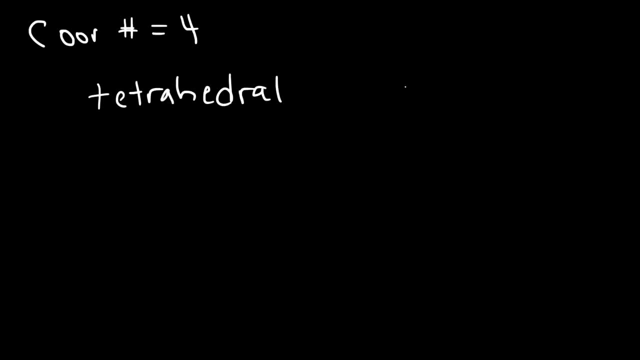 tetrahedral geometry. Another one is the square planar geometry. so the tetrahedral geometry looks something like this, or can have a square plane geometry which looks like this. so if you have a coordination number for the geometry could be any one of those two. so keep that in mind. now, 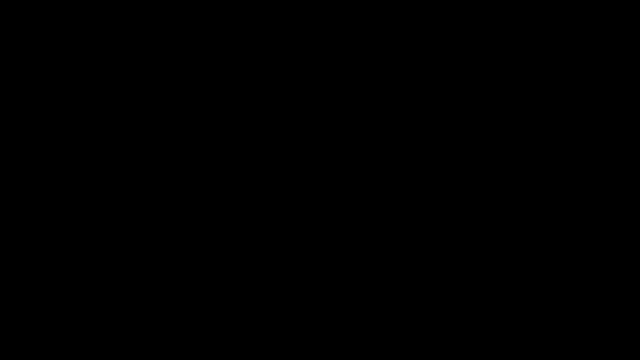 let's talk about the coordination numbers for certain transition metal ions. now let's say, if we have a transition metal ion with a charge of plus one, such as copper plus or AG plus, the coordination number of copper plus one is two and four. for silver it's only two, and so if the charge is low, the 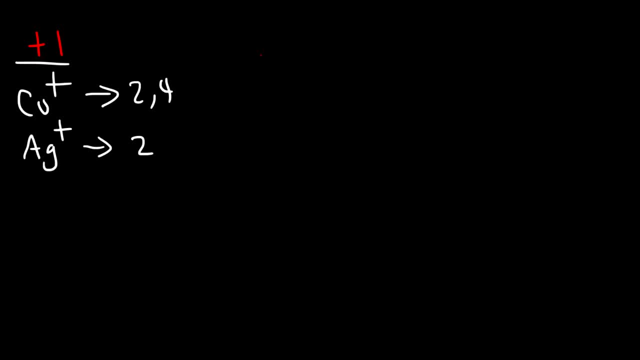 coordination number is relatively low. but notice what happens if we increase the charge. let's say two plus two, so cobalt, for example, the cobalt two plus nine can have a coordination number of four or six. nickel two plus is the same, fe two plus can be up to six and zinc two plus can. 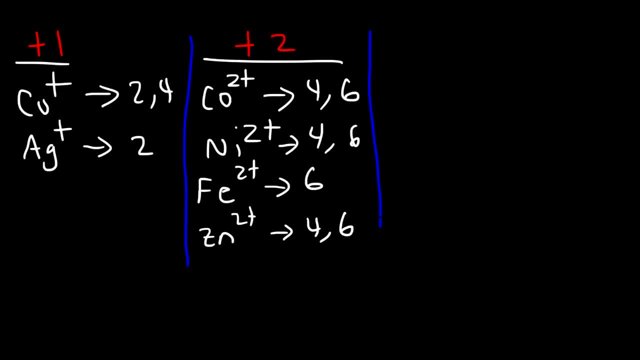 be 4 or 6. now let's look at the plus-three ion. one example is gold 3 plus, which has a coordination number of 4, chromium 3 plus has a coordination number of 6, and cobalt 3 plus has a coordination number of 6.. So notice the 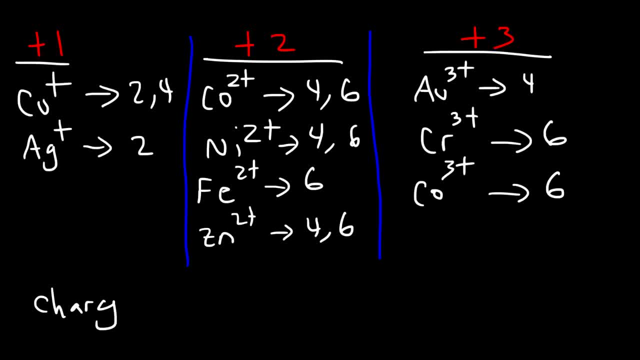 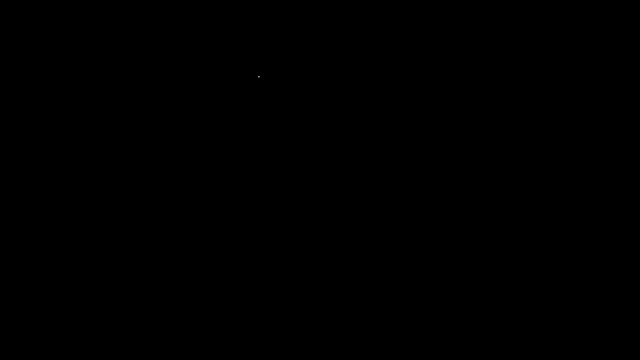 general trend. As the charge on the transition metal ion increases, the coordination number generally increases. And it makes sense, because if a metal ion has a very high charge, it makes sense that it can bind to more ligands. Now you need to be familiar with the different types of ligands. The first 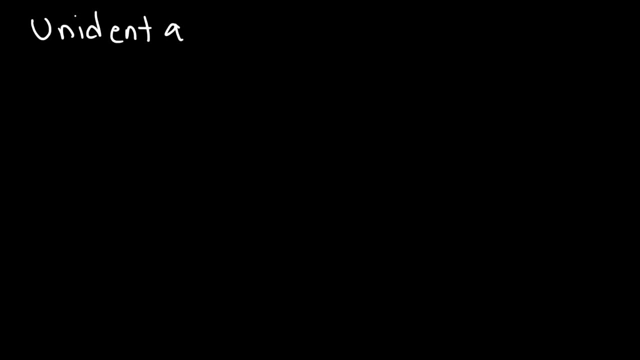 type is called a unidentate, also known as a monodentate ligand, So uni and mono is associated with the number 1. So this tells us that the ligand can only make one interaction with the monodentate ligand. 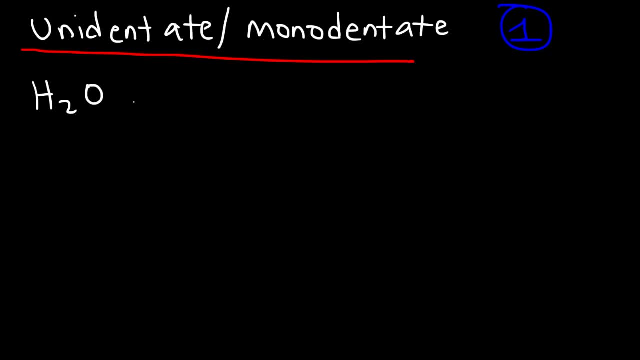 So this tells us that the ligand can only make one interaction with the metal ion. Some good examples of these types of ligands are water, ammonia, chloride, cyanide, thiocyanate, just to name a few. So in the case of ammonia, it has. 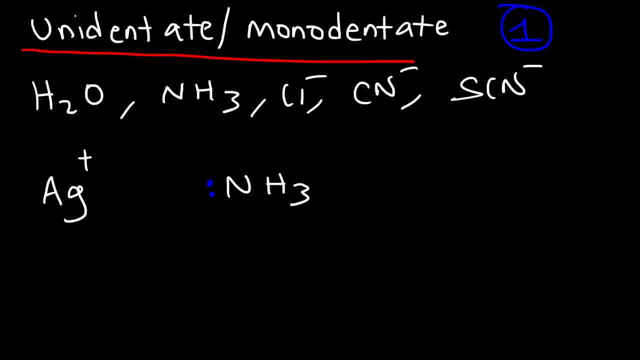 one lone pair, And so it can only form one interaction per molecule with a transition metal ion. A bidentate ligand can only make one interaction with a transition metal ion, So it can only form one interaction per molecule with a transition metal ion. A single iodide ligand can only Martian. 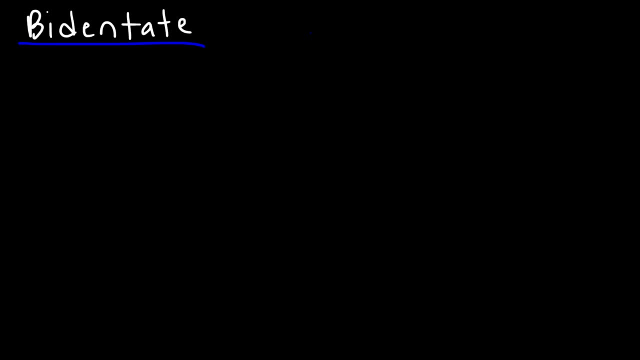 ion. So that's the one example of the monodentate ligand. It can have two interactions per molecule, And the bidentate ligand can only form one interaction per molecule. So when you start looking for an oxygen atom, we're going to have two. 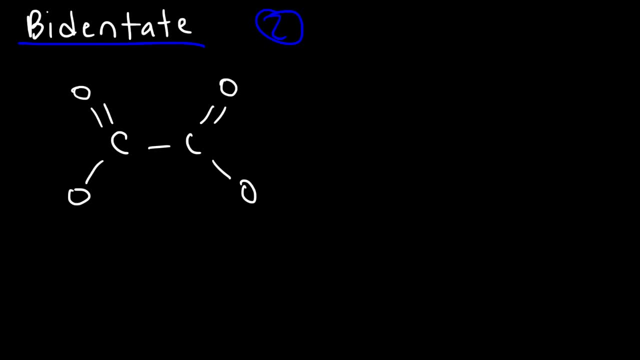 different objects. The monodentate ligand can have two interactions per molecule. Bi is associated with the number 2.. So one example is the oxalate ion. It has two tourism atoms with a negative charge, And let's use a zinc metal cation. that's good for the oxidation. 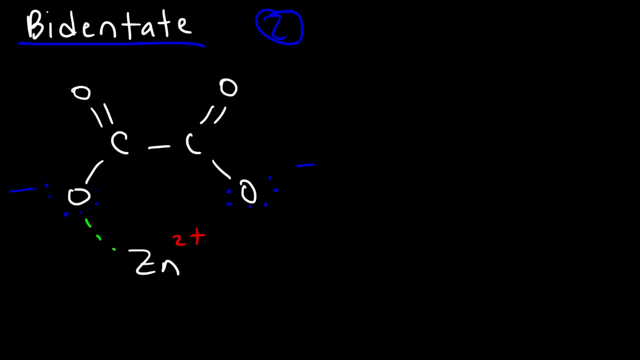 so this is one interaction and that's another. so there's two interactions per molecule, which makes it a bidentate ligand. Another example is ethylene diamine, which you can abbreviate it as EN. So this particular ligand can also make two interactions. 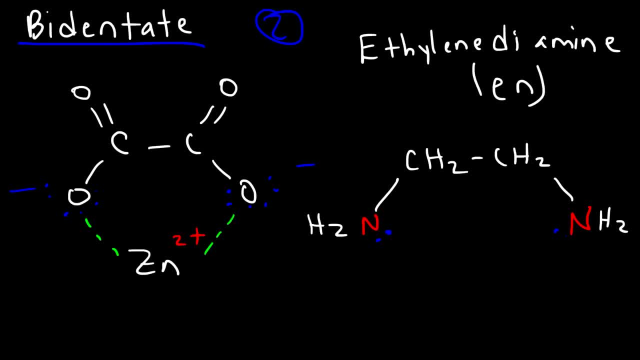 Each nitrogen atom has one lone pair which combined with a transition metal cation. So this is one interaction and this is the second interaction, so that makes ethylene diamine a bidentate ligand. So this is the first interaction and we can also make two interactions, so there's two. 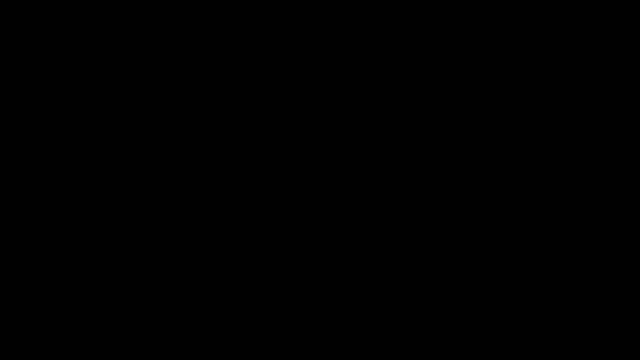 And those are known as chelating ligands. A chelating ligand can interact with a metal ion in more than one way, So bidentate ligands are chelating ligands. Now let's talk about coordination compounds, And here is an example. 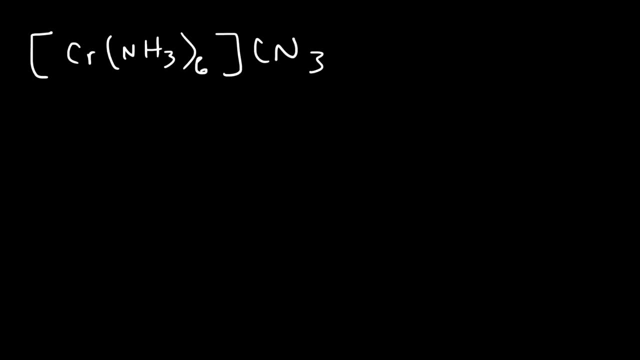 A coordination compound is neutral overall, but it consists of a complex ion and a counter ion. What do you think is the complex ion in this example? Well, you can clearly see it. It's in brackets in this particular example, And so it's Cr 6.. 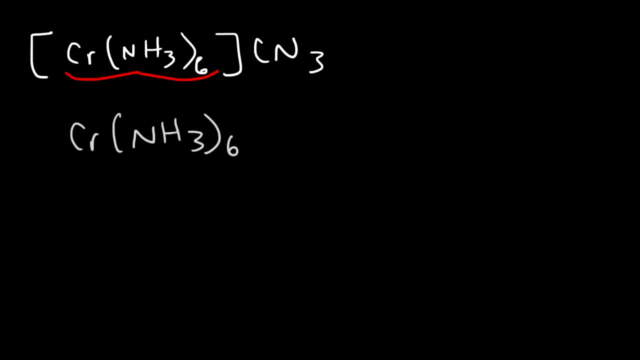 Now, what do you think the charge or the oxidation state of chromium is in this example? Now we know that science. We know that cyanide has to be the counter ion. It's there to balance the charge on chromium And there's three of them, which indicates that chromium has to have a plus three charge. 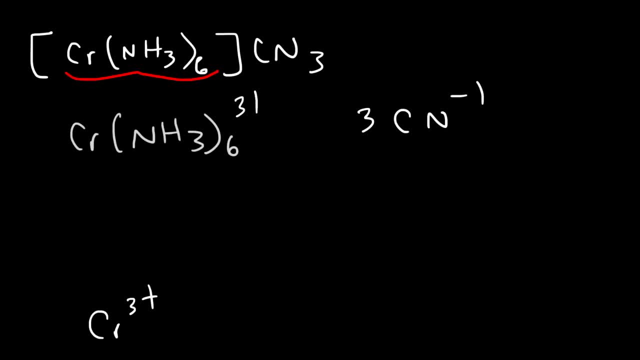 So this particular complex ion has a positive three charge. So this is the complex ion And in this example this is known as the counter ion. The counter ion is the ion that has a positive three charge. The counter ion is the ion that has a positive three charge. 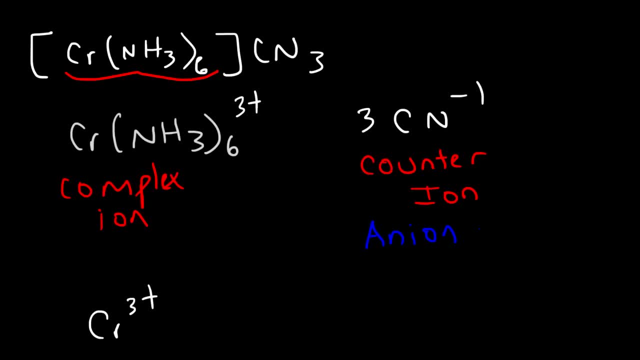 The counter ion that we have in this example is negatively charged, So it's called an anion. But it doesn't always have to be an anion, It can be a cation. In this example, the complex ion is the cation. 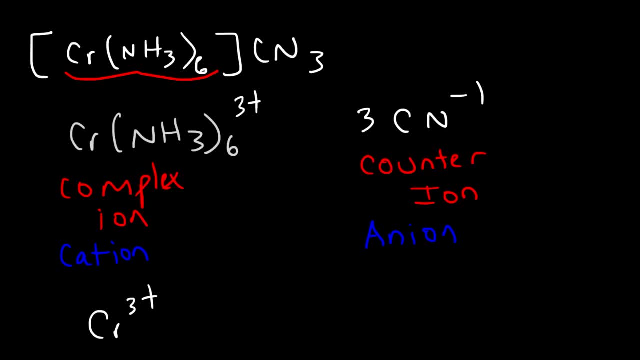 And so the counter ion has to be an anion. But sometimes the roles can be reversed, Like in this example: K3FeCN6.. So in this example we have an anion. So this is the cation And this has to be the anion.